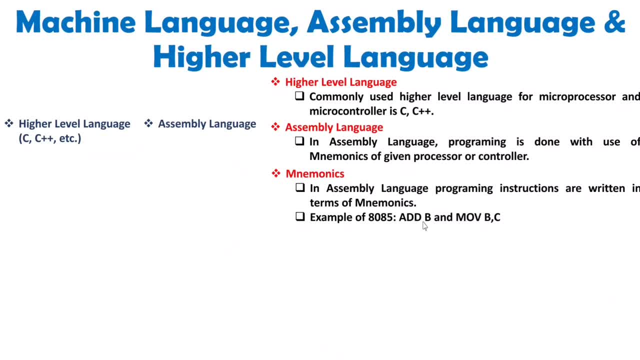 for operation of addition of accumulator and B. When you write mnemonics move B, comma C, it indicates you will be moving data of C into B. So mnemonics explains you the codeword of instructions For different microprocessor and microcontroller. different mnemonics are there right? Let me explain you all those. 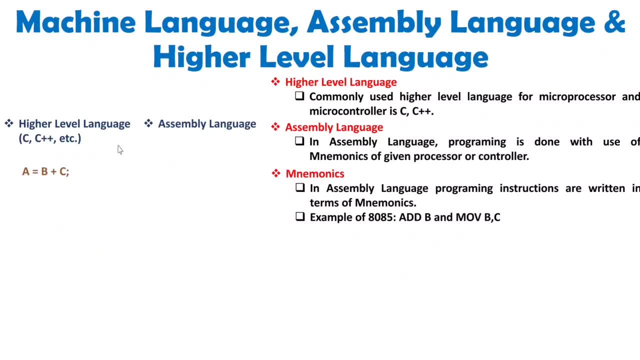 things by practical example, so that will be more clear. So let us say we are talking about higher level language. So in C CPP we can directly write: A is equals to B plus C, right, So what it does, It will be adding B to C. So let us say we are talking about 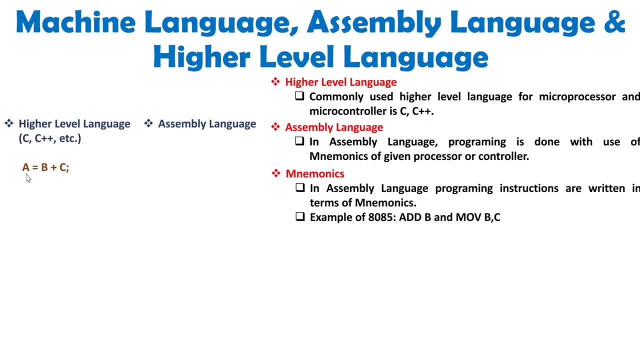 B and C and answer will get stored in A. But when you want to do this operation in assembly language, at that time you will have to write assembly code based on mnemonics. So I will show you one practical example. You see, move A, comma B: that is written. 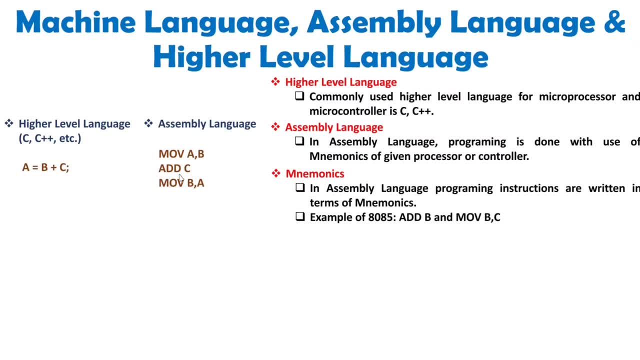 What it means B is going inside A. After that add C is written. What it means C will get added with A and answer will get stored in A. After that, again I have written move B, comma A. What it means A will get transferred into B. So that is how we are writing instructions. 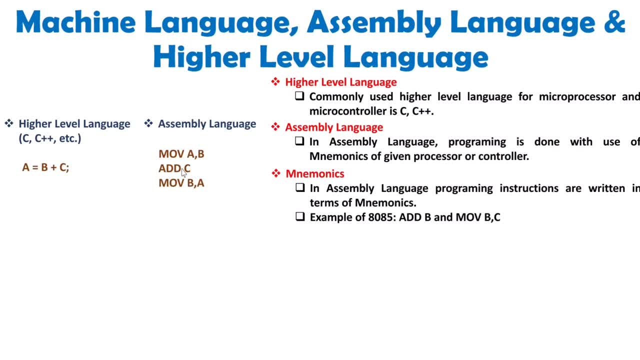 by mnemonics And this is what assembly language that you can see And this assembly language mnemonics are different for different microprocessor and microcontroller. Here we are talking about 8085 microprocessor, So with that, these are the mnemonics which are available Now. 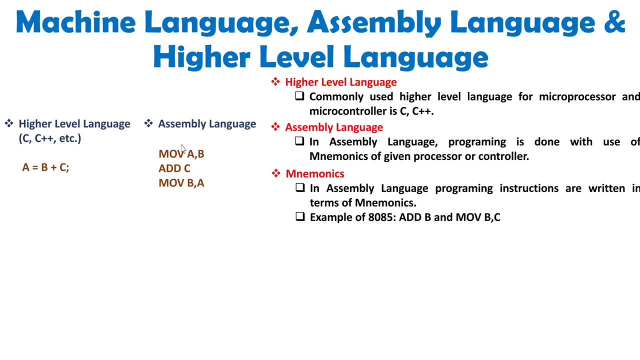 my job is to explain you what is machine learning, What is machine language? So you cannot have directly machine language Here. there is a need of compiler and assembler, My dear students, here when we talk about higher level language, so higher level language that can be converted into machine language by using compiler. 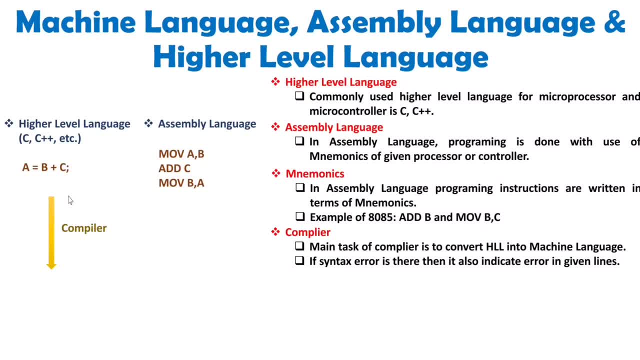 So main job of compiler is to convert higher level language into machine code or machine language. And compiler will also show you errors when you write syntax error right. So compiler job that is to convert higher level language into machine language. And when we talk about assembler, then assembler is converting assembly language into machine. 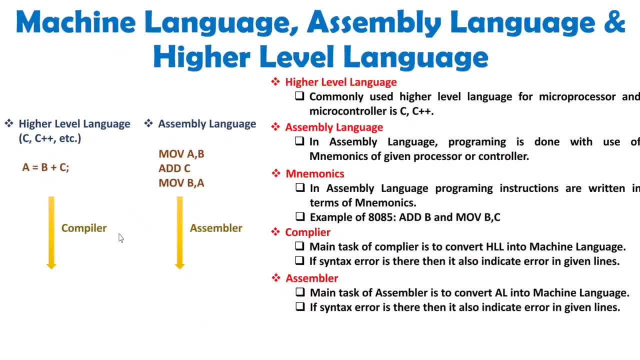 language. So, my dear students, assembler job is similar to compiler. Only thing is, when you write code in compiler Assembly language, at a time, assembler will convert this assembly language into machine language and assembler even can show you error, as if there is syntax error or some logical 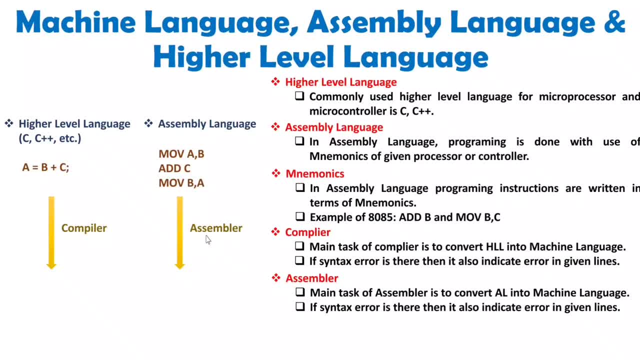 error, But you should know in the interview there are questions that is coming many times like: can you explain me what is compiler? So its job is to convert higher level language into machine language and assembler's job is to convert assembly language into machine language. 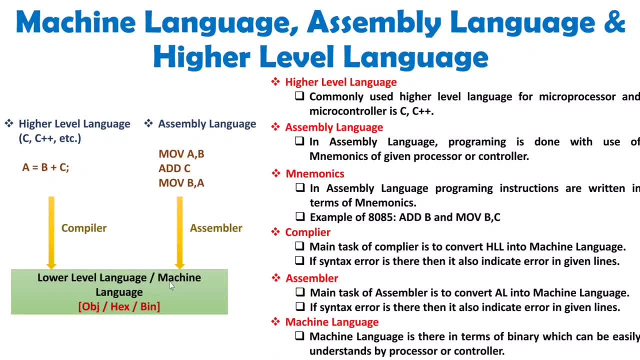 Now, my dear students, what is machine language? So, dear students, machine language is lower level language that is there in terms of binary See microprocessor cannot understand this higher level language or assembly language. It only understands things based on binary 1010 data. 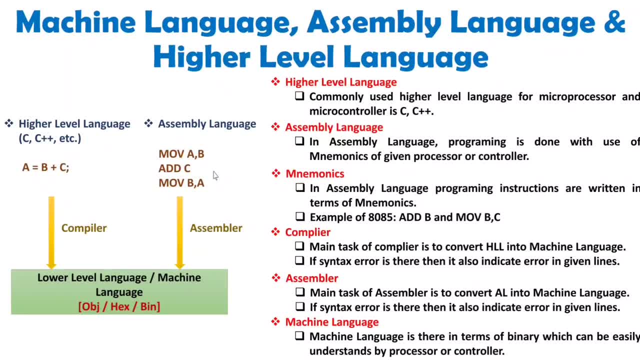 So what we do is we convert these programs in terms of binary code, And that binary code is referred as machine language, right? The reason is we cannot even remember how 1010 that we need to write with respect to different instructions, right? 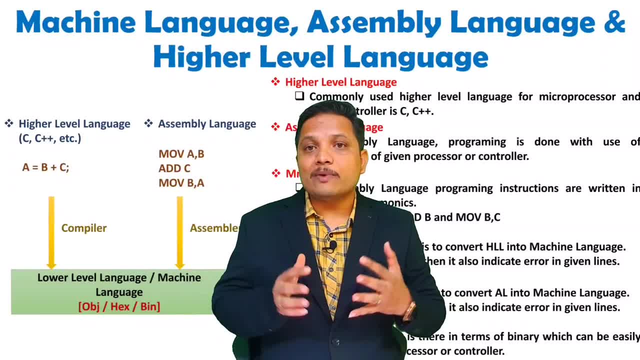 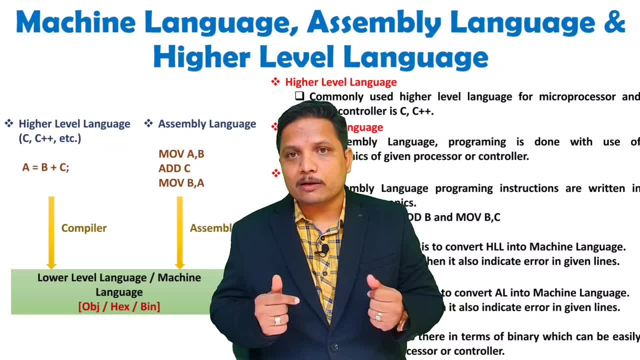 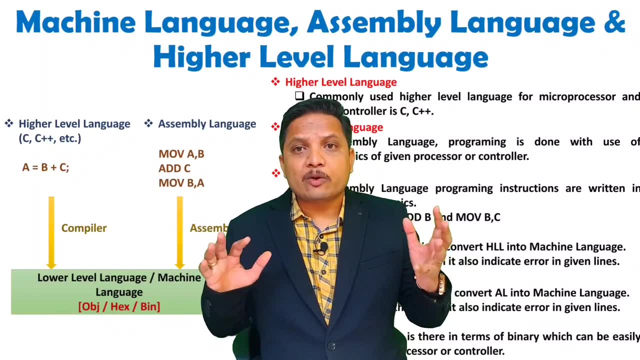 So, my dear students here, what we do here, we write programs in assembly language with 8085.. But as if you want to program AVR microcontroller, then there are many instructions, And if you want to operate with 5 to 7 different microprocessor or microcontroller, then is. 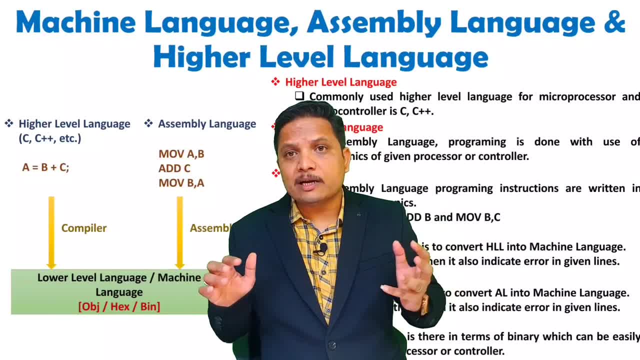 it possible that you can remember instructions for that many processor and controller? Simply no right. So what you do is you learn only a few languages, like C CPP. So by using C CPP, we can be able to program in a single way. 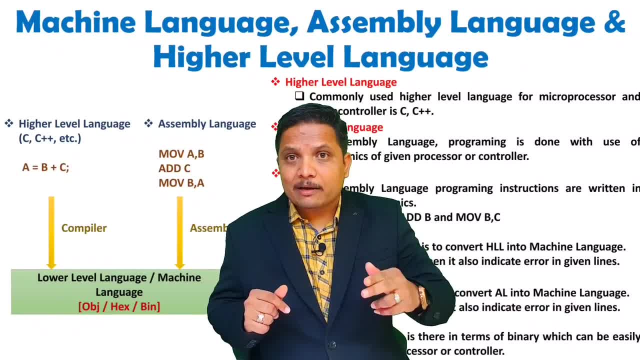 And by using that single way, by using compiler, we convert that C language code into C language. And by using that single way, we convert that C language code into C language code. And by using that single way, we convert that C language code into C language code. 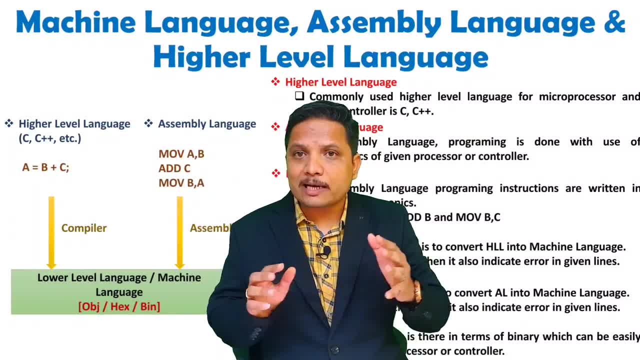 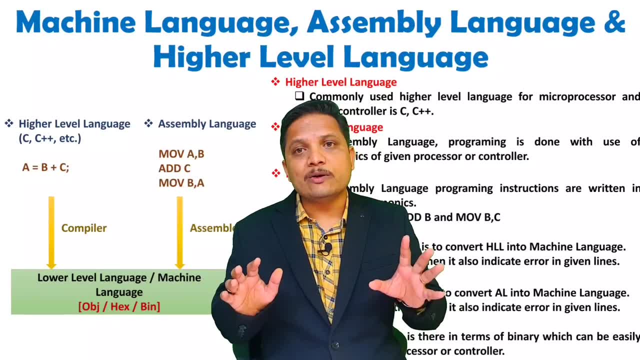 And by using that single way we convert that C language code into machine code. Machine code is always there in terms of binary. The reason is: microprocessor and microcontroller does not understand any other thing than zeros and ones Here. why don't we write code in terms of machine code? 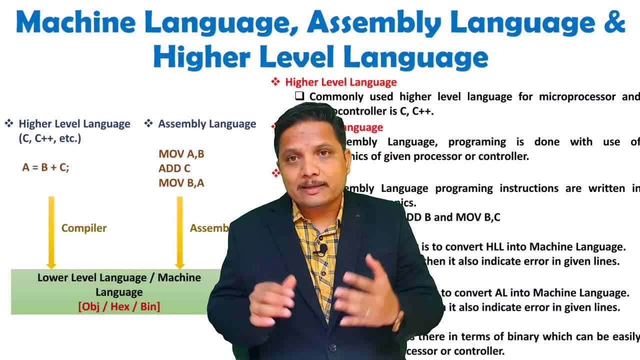 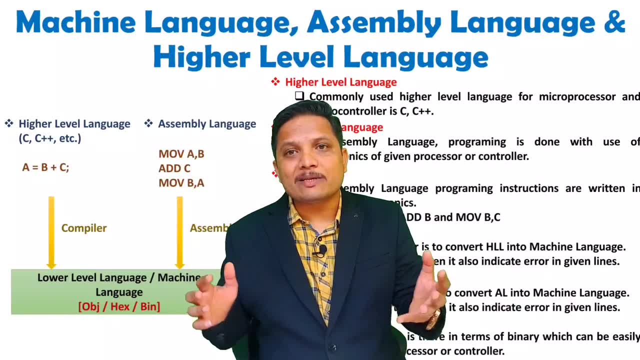 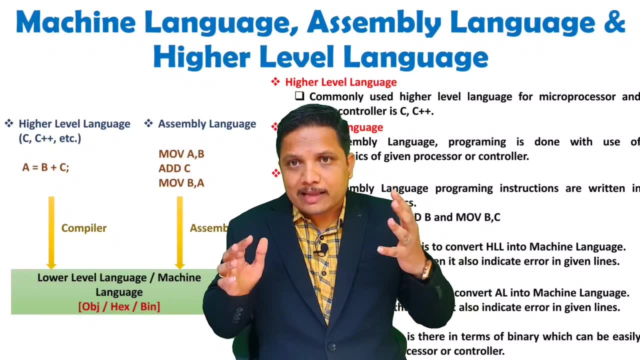 See, you don't write codes in terms of machine code. The reason is it is very complicated to remember that many numbers. How can you remember 0101 sequence for different instructions? You cannot remember sequence of zeros and ones, right? You can understand some mnemonics of assembly language or you can understand programming. 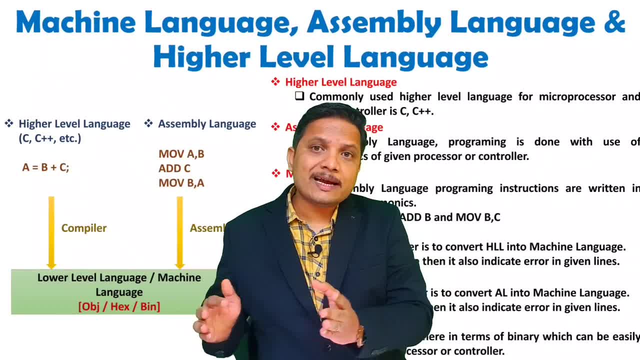 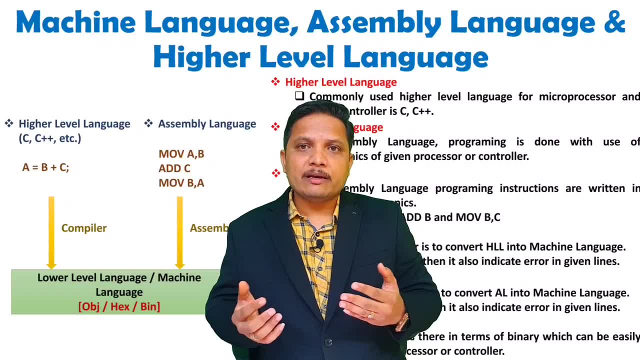 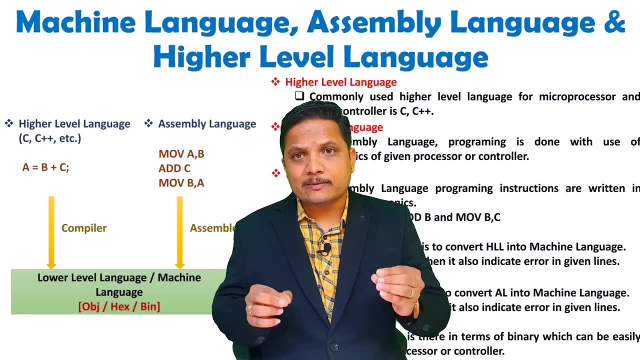 language like C or CPP. If you give efforts in that direction, then you can be able to program many things right. So if you have knowledge about C or CPP, definitely you are eligible to program any microprocessor or microcontroller In that situation. only thing is you will have to understand what is programming model. 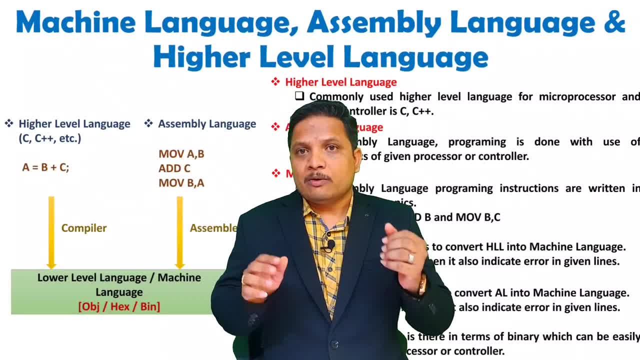 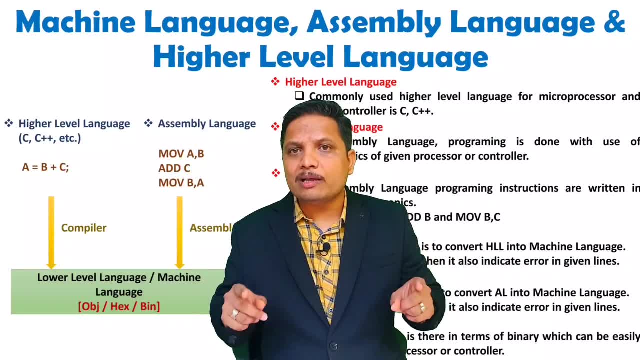 of given microprocessor or microcontroller. Programming model means how many resistors are there which is available for programming purpose. Once you understand that programming model, you can directly start making programs by using C and CPP. So when you go in industries of embedded system, at that time it is very essential that you 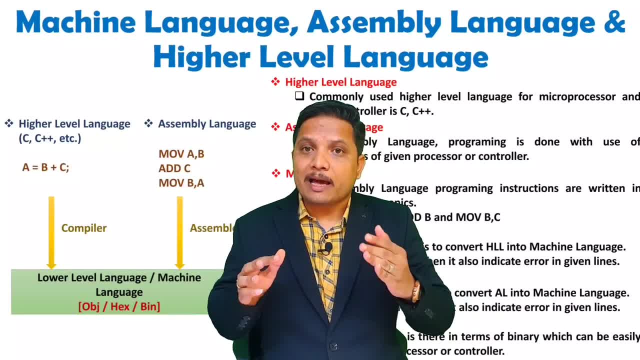 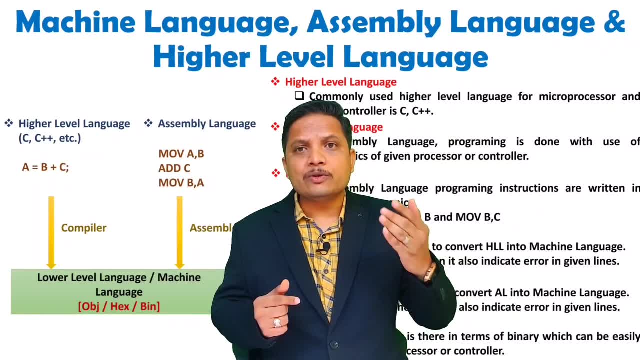 should know C and C++. By having that language, you can be able to program many other embedded devices, right? Only thing is you should know how to compile the code, and whatever errors are there in compiler, you just resolve it and you can load it into processor or controller, right. 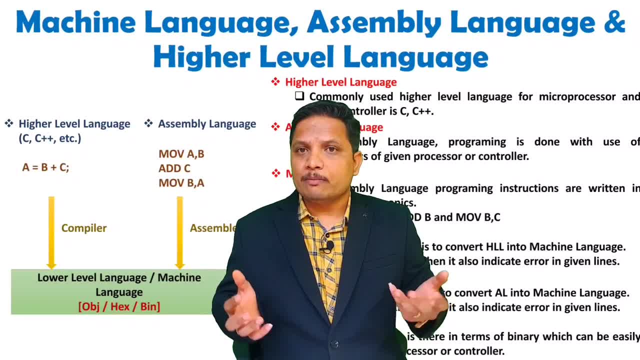 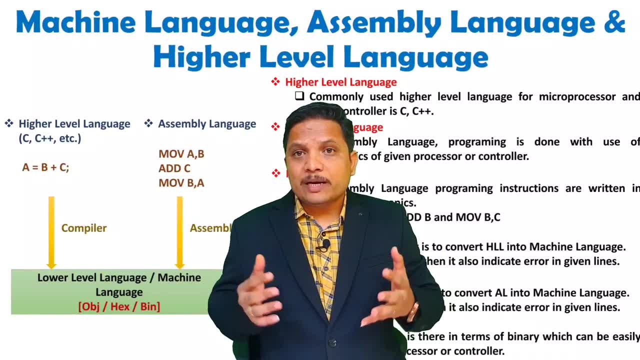 The reason is machine language that could be easily understood by processor or controller. So that is how things are there, with microprocessor as well as microcontroller. This is how it works. This video is, in general, video right, where there are few basic things that you must know. 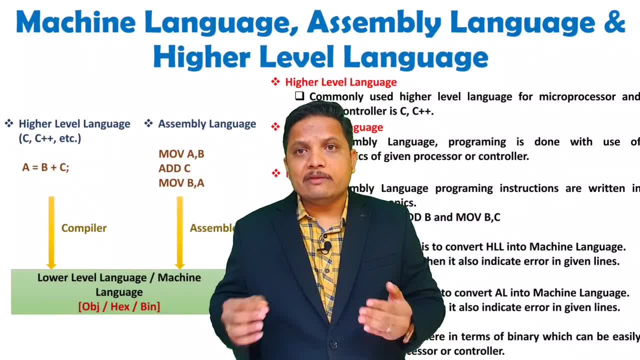 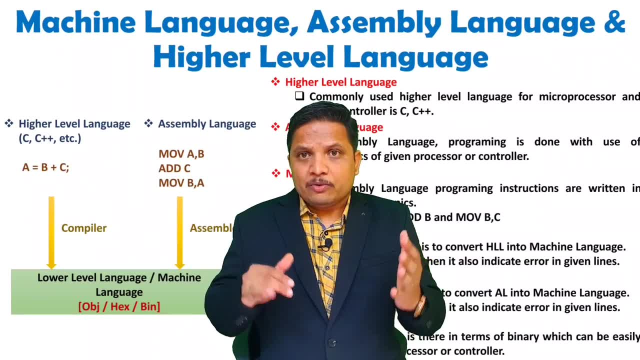 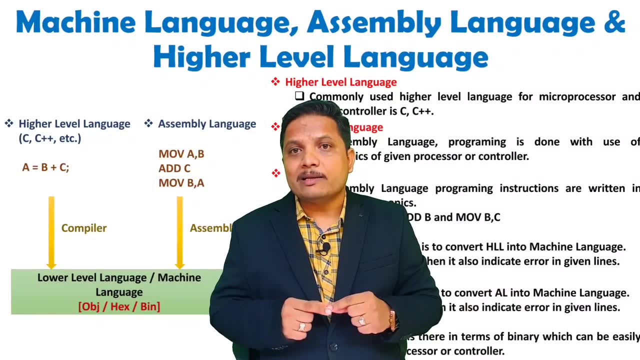 The reason is this world is getting digitized and, in future, many other things that will come in front of you, which is there based on programming, and you will have to train many other things in terms of robotics or automation, in which also these fundamentals are very essential. I hope you have understood this. Thank you so much for watching this video.